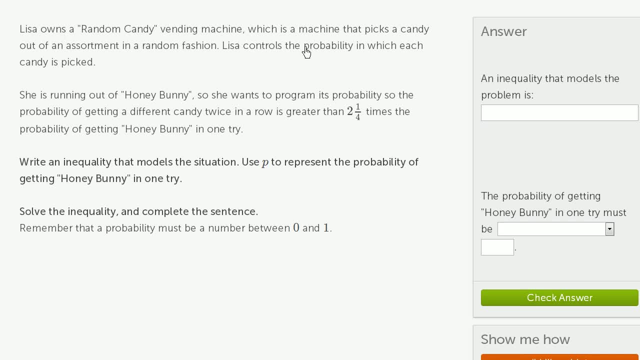 Lisa owns a random candy vending machine, which is a machine that picks a candy out of an assortment in a random fashion. Lisa controls the probability in which each candy is picked. She is running out of Honey Bunny, so she wants to program its probabilities. 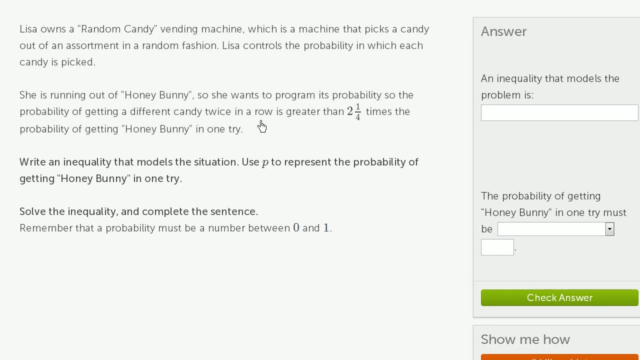 so that the probability of getting a different candy twice in a row is greater than 2 and 1 fourth times the probability of getting Honey Bunny in one try. So let me read that again. She wants to program its probabilities so that the probability of getting a different candy twice. 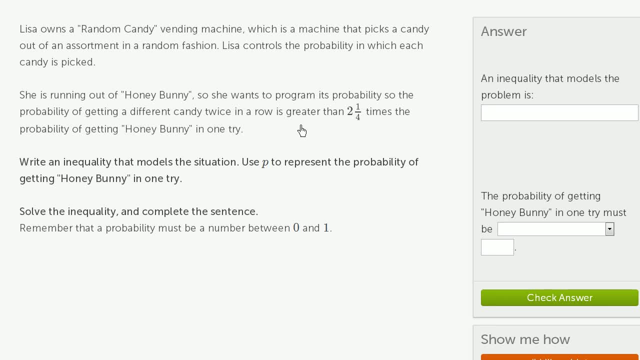 in a row or really any other candy twice in a row is greater than 2 and 1 fourth times the probability of getting Honey Bunny in one try. Write an inequality that models the situation. Use p to represent the probability of getting Honey Bunny in one try. 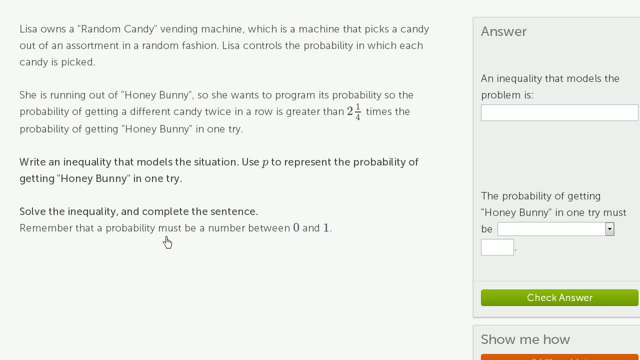 Solve the inequality and complete the sentence. Remember that the probability must be a number between 0 and 1.. So we want to write the inequality that models the problem here, And then we want to complete the sentence. The probability of getting Honey Bunny in one try must be: 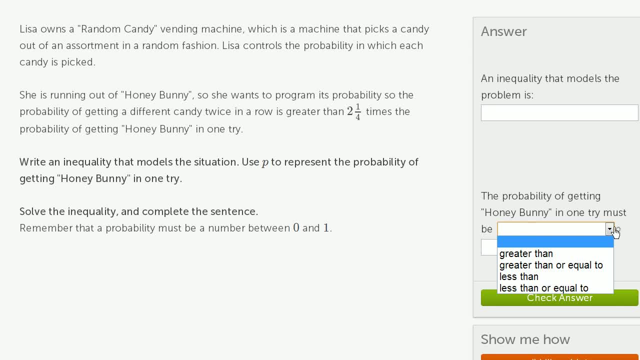 so they give us a bunch of options: greater than, greater than or equal to, less than, less than or equal to- And then we have to put some number here. So to work through this, I've copy and pasted this problem. 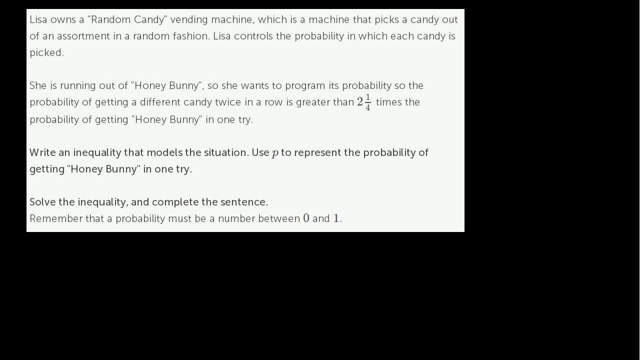 onto my little scratch pad right over here, And so let's just think about it a little bit. So they tell us: use p to represent the probability of getting Honey Bunny in one try, And they also say she wants to program this probability so that the probability 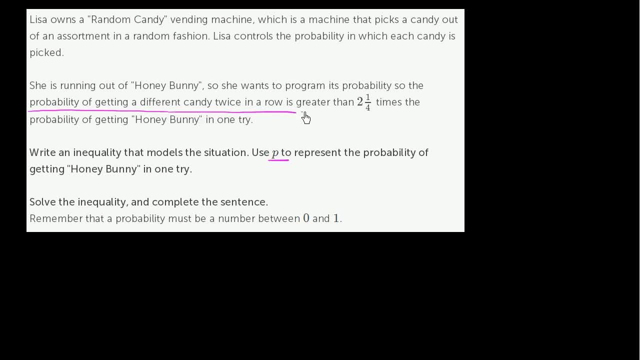 of getting a different candy twice in a row is greater than 2 and 1. fourth, the probability of getting Honey Bunny in one try. So if p is the probability of getting Honey Bunny, what's the probability of getting any other candy at once? 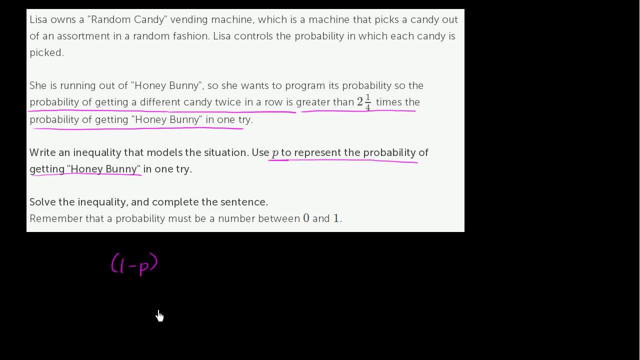 Well, that's going to be 1 minus p. If you have a probability of p of getting Honey Bunny, well then it's 1 minus p, 1 minus p of anything but Honey Bunny. Now, what's the probability of getting this twice in a row? 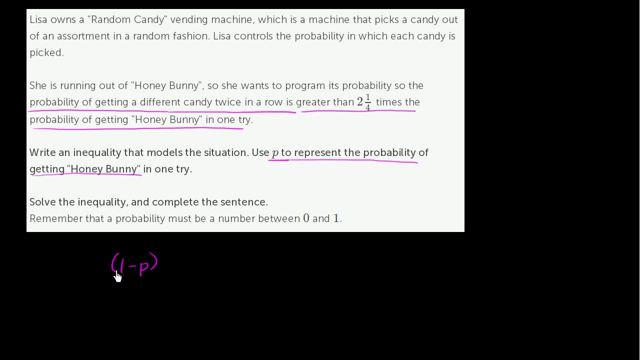 of getting anything else twice in a row. Well, you're just going to multiply this probability times itself. It's going to be 1 minus p times 1 minus p, Or we could just write that as 1 minus p squared. So this right over here is the probability. 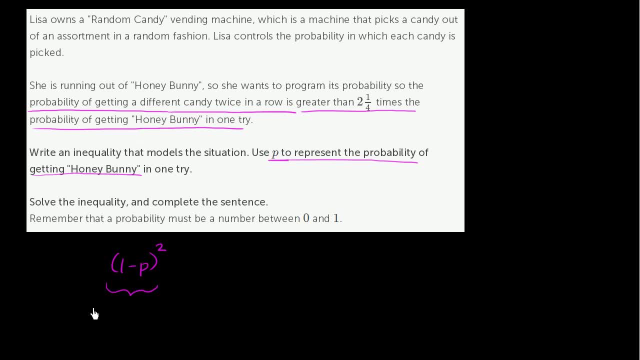 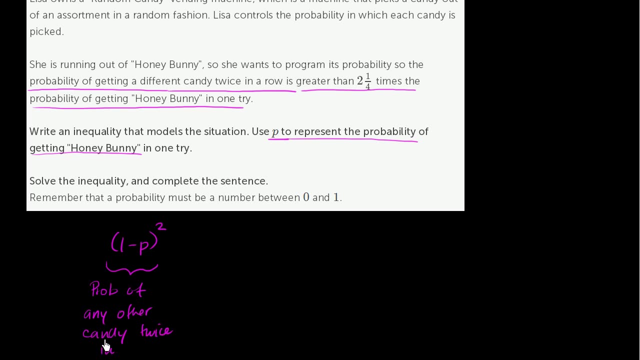 of getting a different candy, any other candy, twice in a row. So prob of any. Any other candy, Any other candy, Any other non-Honey Bunny candy, any other candy twice in a row. Now they tell us that this probability 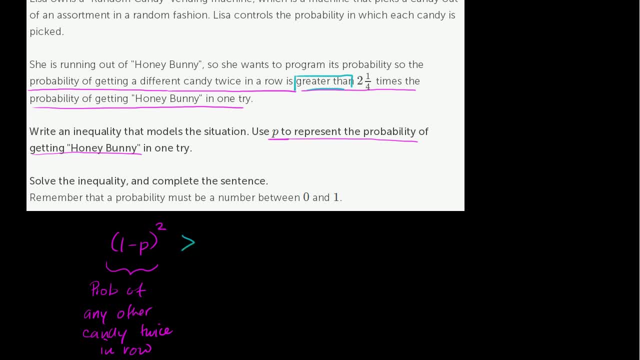 needs to be greater than 2 and 1 fourth times the probability of getting Honey Bunny in one try. So it's greater than 2 and 1 fourth. 2 and 1 fourth times the probability of getting Honey Bunny in one try. well, that is p. 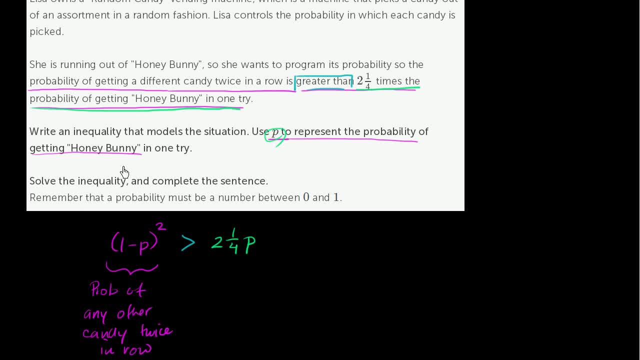 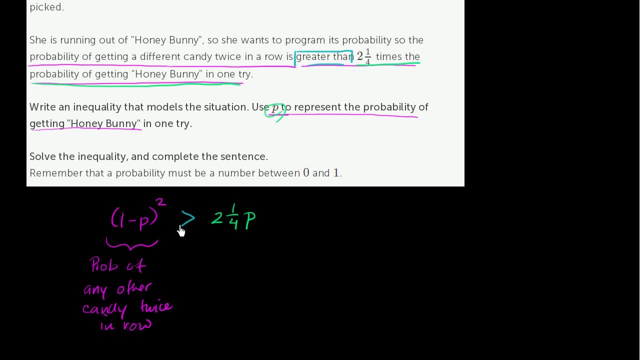 So we have just set up the first part. We have written an inequality that models the situation. Now let's actually solve this inequality, And so to do that, I will just expand: 1 minus p squared out- 1 minus p squared is the same thing as p squared. 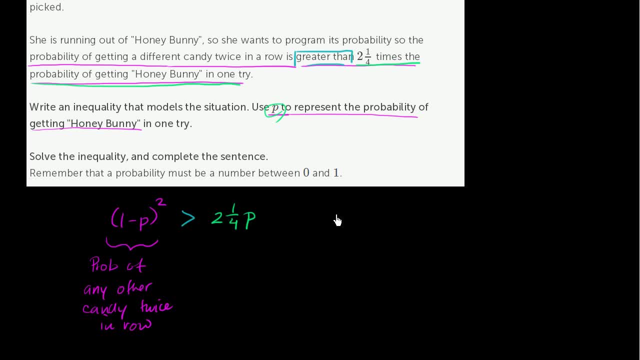 It's the same thing as the same. Well, I'll just multiply it out. So this is going to be 1 squared, 1 squared minus 2p, plus p squared, And that's going to be greater than 2 and 1. fourth p: 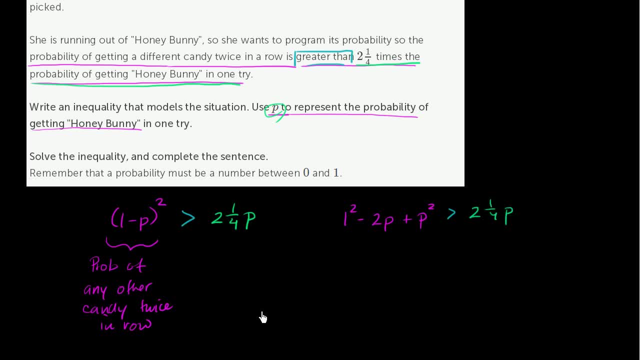 Greater than 2 and 1 fourth p. Now let's see: If we subtract 2 and 1 fourth p from both sides, we're going to be left with- and I'm going to reorder this- we're going to get p squared. 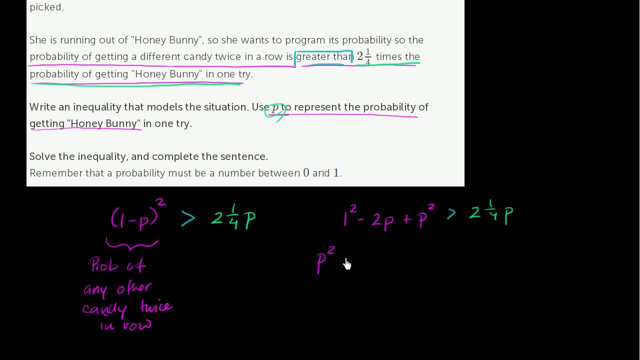 So you have minus 2p, minus 2 and 1 fourth p. So that's going to get us minus 4 and 1 fourth p. Or let me just write that, as 17 over 4p plus 1 is greater than 0.. 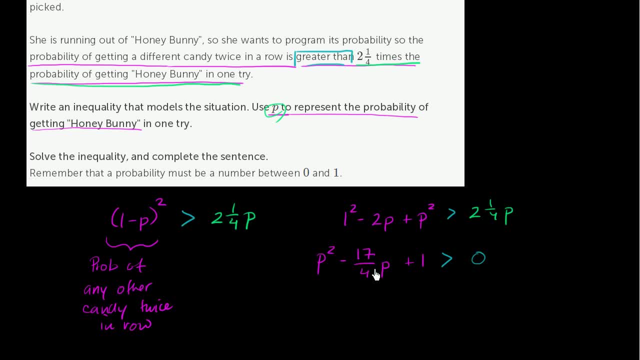 And so let's think about solving this quadratic right over here, And under which circumstances is this greater than 0?? And to think about it, let's factor it. And actually, before we factor it, let's simplify. Let's simplify it a little bit. 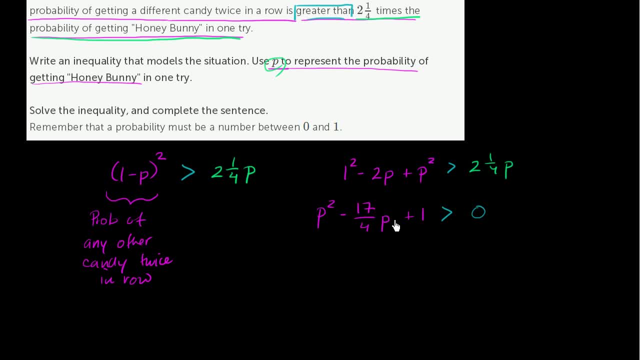 I don't like having this 17 fourths right over here, So let's multiply both sides times 4.. And since 4 is a positive number, it's not going to change the direction of this inequality, So we could rewrite this as 4p squared minus 17p plus 4. 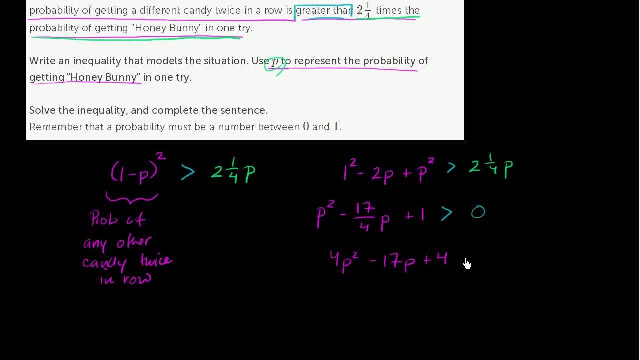 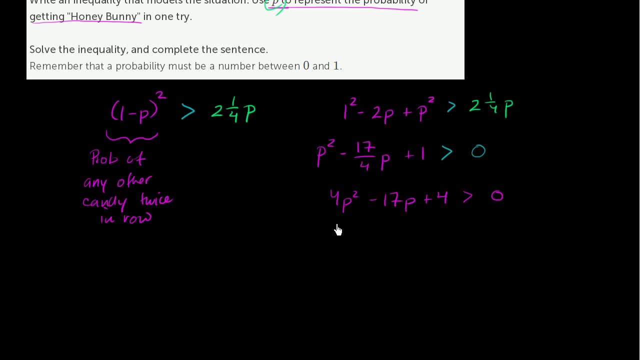 is greater than 0.. And let's see what are the roots of this. And we could use a quadratic If we wanted to do it really quick. we could probably do it other ways But negative b. so it's going to be 17 plus or minus. 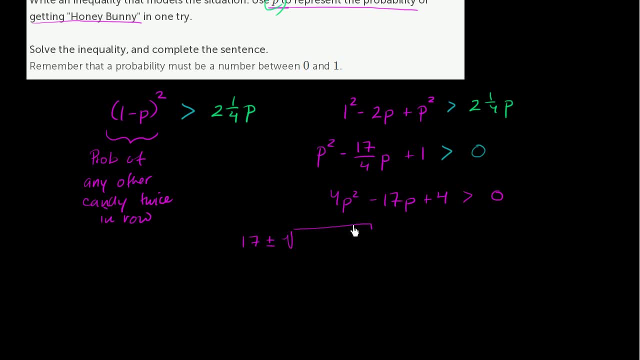 the square root of negative. 17 squared b squared, So that's 289 minus 4 times a times c. Well, a times c is 16 times 4, so minus 64.. All of that over 2 times a. 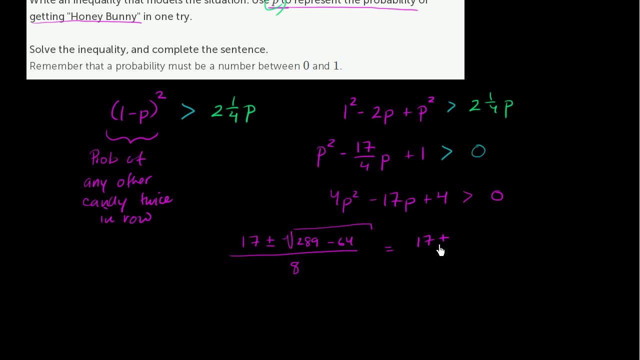 All of that over 8.. So that's 17 plus or minus. let's see, this is the square root of 225 over 8,, which is equal to 17 plus or minus 15 over 8, which is equal to, let's see, 17 minus 15 over 8. 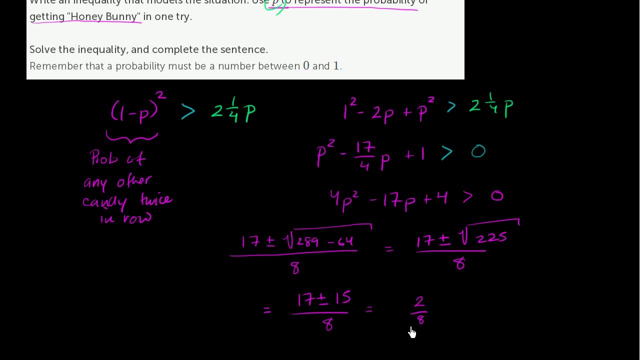 is 2 eighths, which is equal to 2 eighths or 1 fourth. So that's one of them. That's when we take the minus And if we add 17.. 17 plus 15, that gets us to 32. divided by 8 is 4, or 4.. 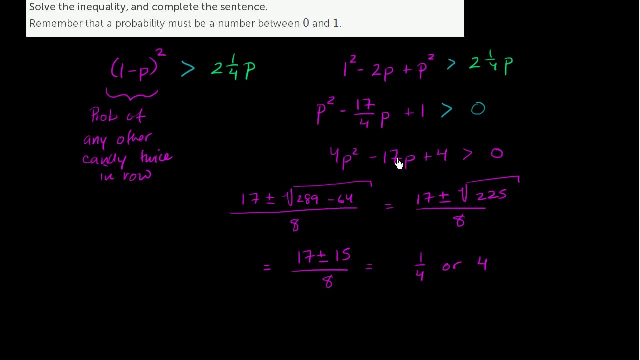 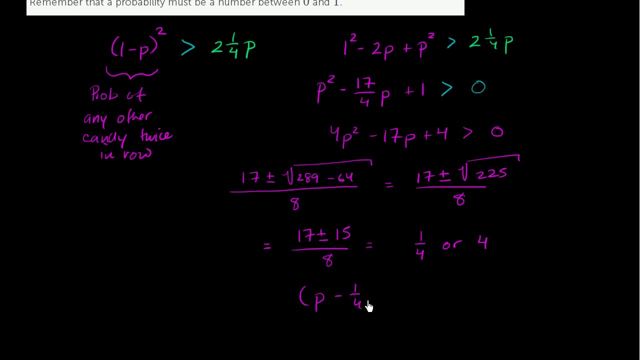 So there's two situations right over here, So let's factor this out. We could write this as p minus 1. fourth times, p minus 4 is greater than 0. So under what circumstances is this going to be true? What constraints are this going to be true? 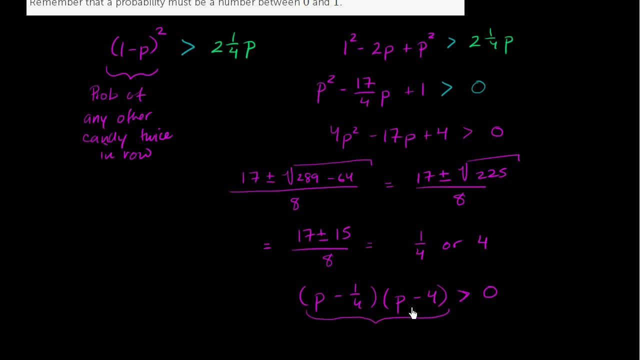 Well, if you're taking the product of two terms, and they are going to be greater than 0, that means that these two things have to be the same sign, Or actually, in particular, they both have to be positive or they both have to be negative. 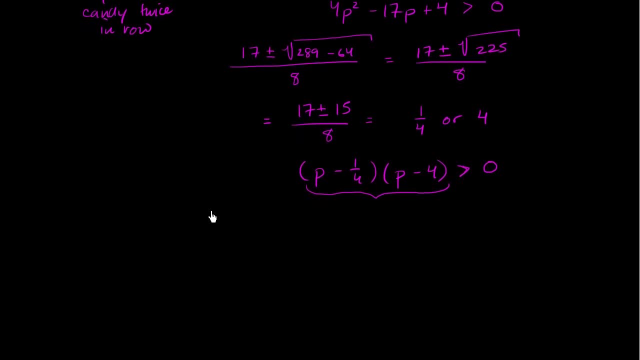 So let's look at those two situations, So I'll switch colors here just for fun. So both positive or both negative. So if they're both positive, that means that p minus 1, fourth, has to be greater than 0.. And p minus 4 is greater than 0. 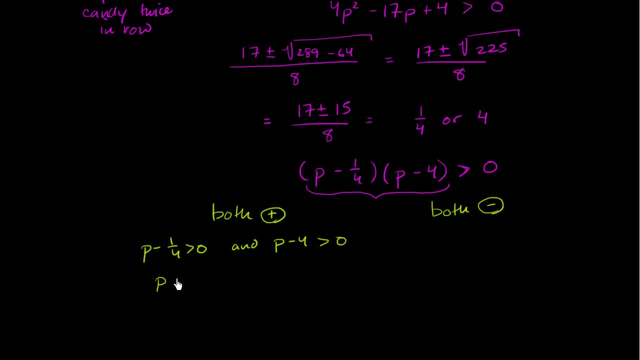 Add 1 fourth on both sides right over here You get p is greater than 1. fourth, p is greater than 4.. So that's the situation where they are both positive. Now what about if they're both negative? Well then you have p minus 1. fourth is less than 0.. 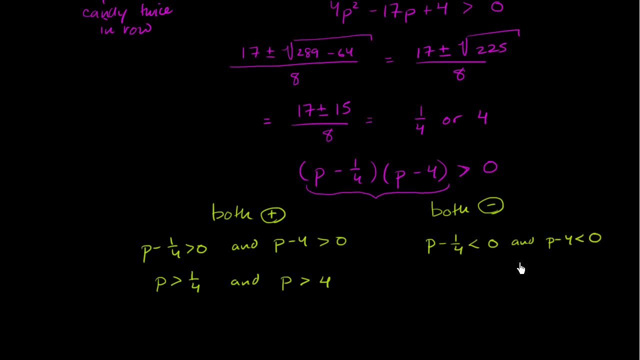 And p minus 4 is less than 0. Add 1 fourth here. So p needs to be less than 1 fourth And p needs to be greater than 0. It needs to be less than 4.. Now, what does this constraint simplify to? 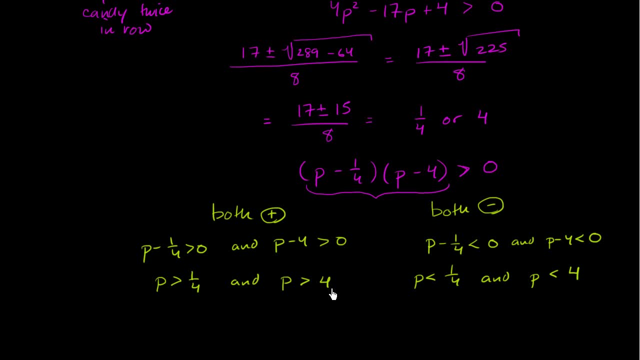 p has to be greater than 1 fourth And p has to be greater than 4.. Well, if p is greater than 4, it's definitely going to be greater than 1 fourth. So all of this collapses into p needs to be greater than 4.. 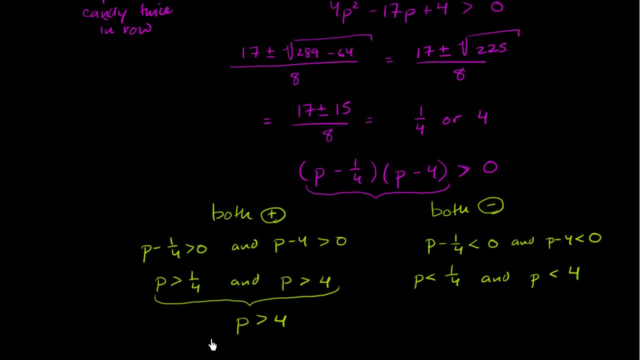 That's the situation. where both are positive, p must be greater than 4.. Now, what about here? Well, if p is less than 1 fourth, it's definitely going to be less than 4.. And this is an and right over here. 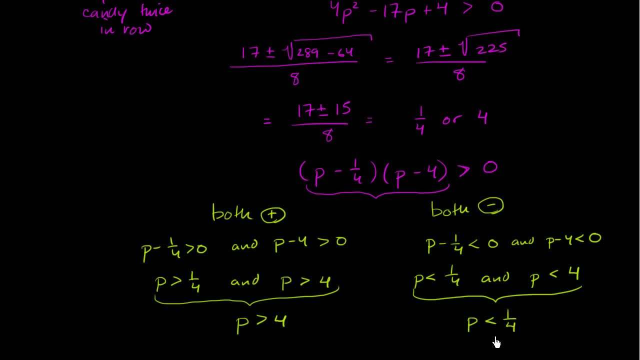 So this collapses to: p is less than 1 fourth. So which one do we go with? p needs to be greater than 4, or p needs to be less than 1 fourth. Well, we need to remind ourselves that we're talking about a probability. 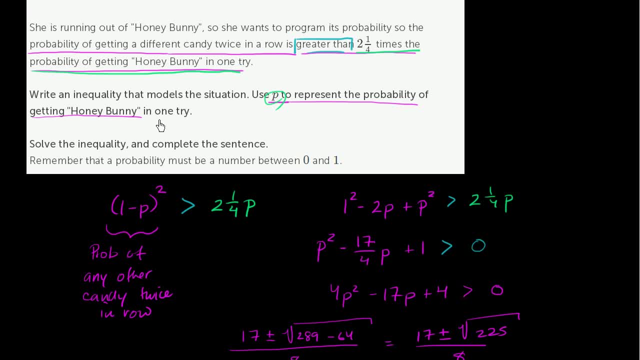 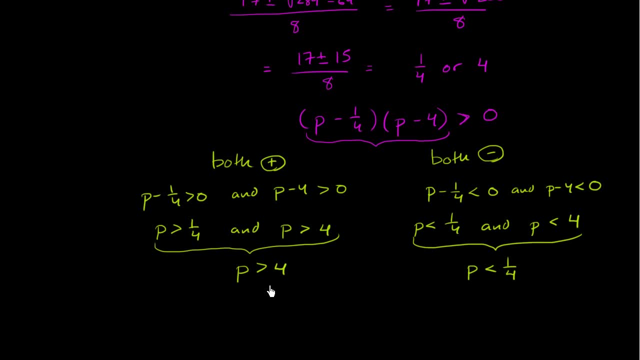 To go back to the original problem, we're talking about a probability of someone getting honey bunny in one try. The probability must be between 0 and 1.. So the probability having to be greater than 4, well, that just doesn't make any sense.